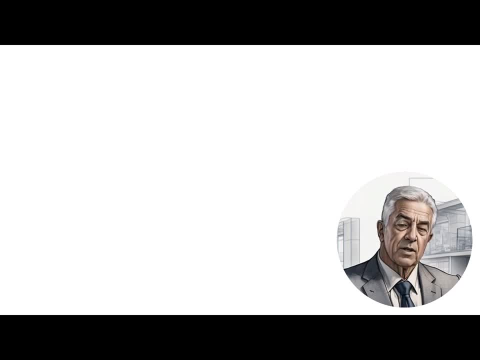 Welcome to the world of structural analysis. Whether you're an engineer, architect or simply have a fascination with building design, this video is for you. Today, we'll be exploring the three main types of structural analysis programs: elastic plastic and elastic plastic. 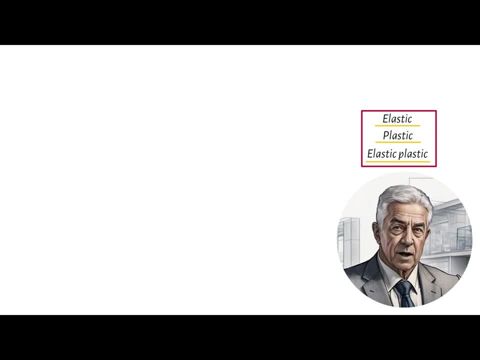 Interestingly, do you ever wonder how the structures you see around you can withstand the forces of nature and everyday life? Well, that's where these programs come in. They calculate the forces acting on a structure and help determine its ability to resist collapse. However, it's important to note that these programs do not include checks for the 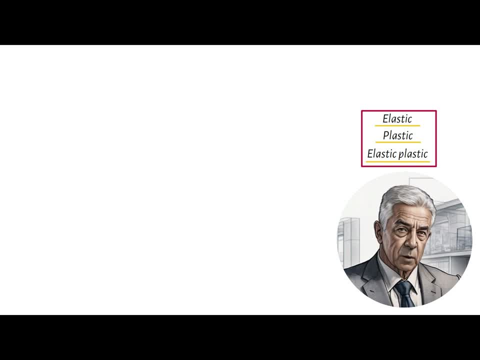 members' ability to sustain the generated forces, which is a separate design activity. Moving on, let's dive into the different types of analysis programs. Elastic analysis, the most common type of analysis, is the type of analysis that is used to determine the forces of nature and everyday life. 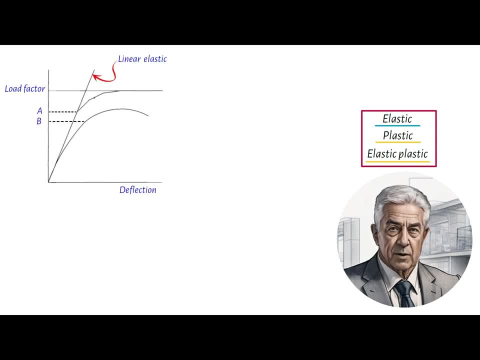 The most commonly used, assumes linear elastic behavior of the material being modelled. It calculates forces but does not account for failure due to yielding or buckling. Conversely, plastic analysis methods determine the set of plastic hinges that form a collapse mechanism under a given set of loaves. Yet this method has mostly been replaced. 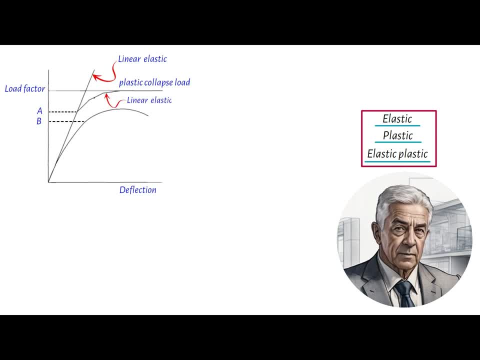 by programs that perform elastic plastic analysis. These programs take into account the formation of plastic hinges and the calculation of defections and bending moments. Additionally, we also have first-order and second-order structural analysis. In first-order analysis, the structure's stiffness is assumed to remain constant and unaltered. 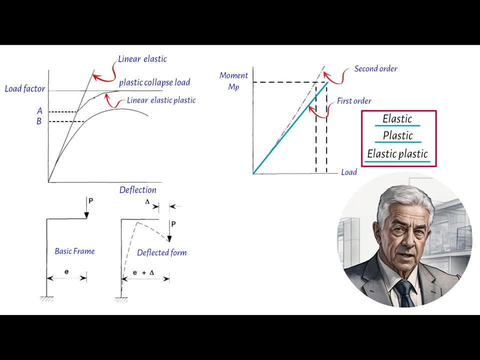 by changes in geometry when loaded. This approach is commonly used for most orthodox steel structures. Conversely, second-order analysis takes into account the changes in effective stiffness of structure due to the loads acting upon it. This is necessary for structures such as cable struts and members in bending. 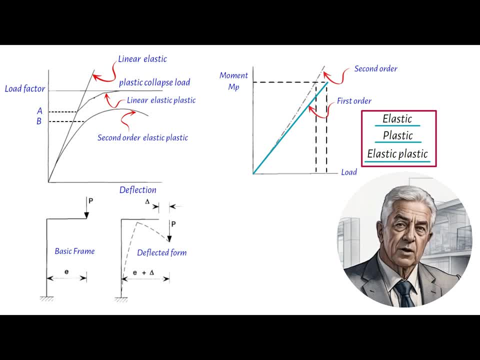 Moreover, in the design of multi-story rigid jointed frames, it is important to take second-order effects into consideration. This can be done by ensuring sufficient stiffness or using the amplified sway method. Conversely, if a multi-story frame has an unorthodox bracing arrangement, second-order effects may be significant and should be checked.